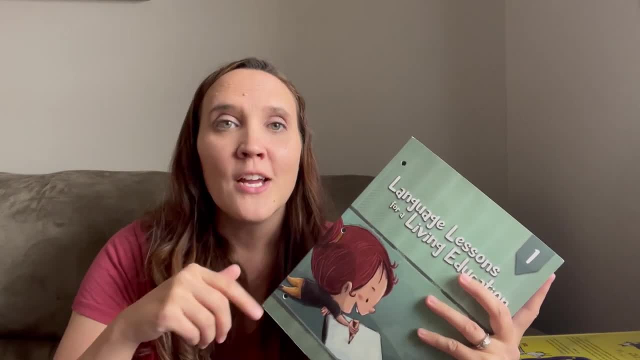 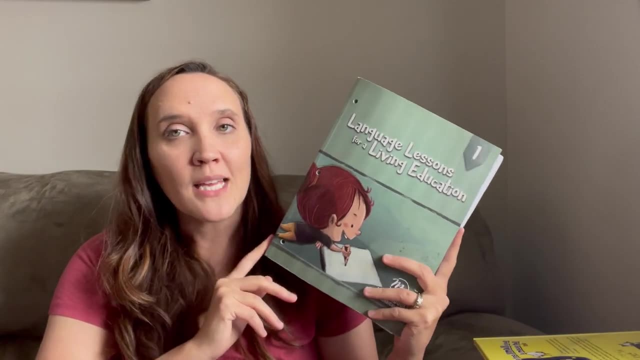 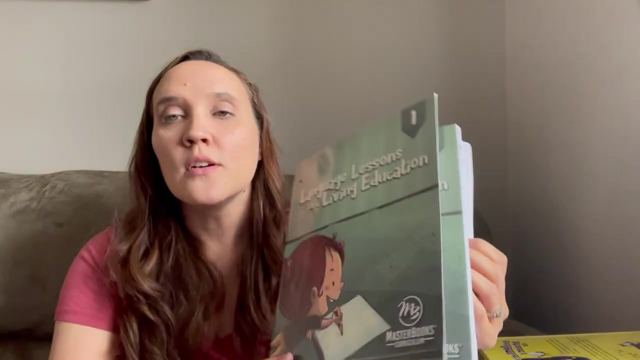 I will link it down below. I did it, I think, last year when I first ordered the curriculum, but we did not start it until this school year. So the curriculum comes like this: It is an open and go all in one. All of the notes that you will need as the teacher are written. 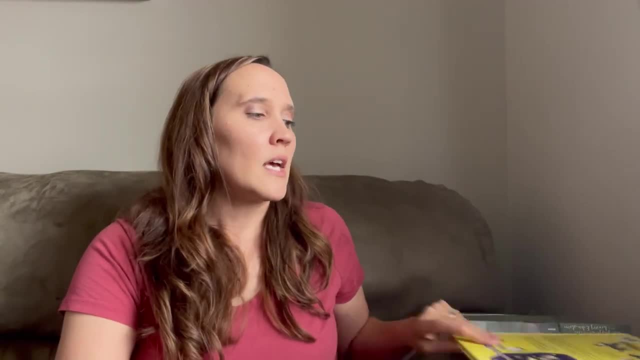 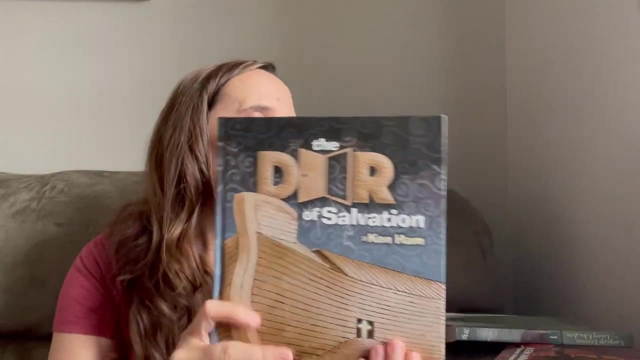 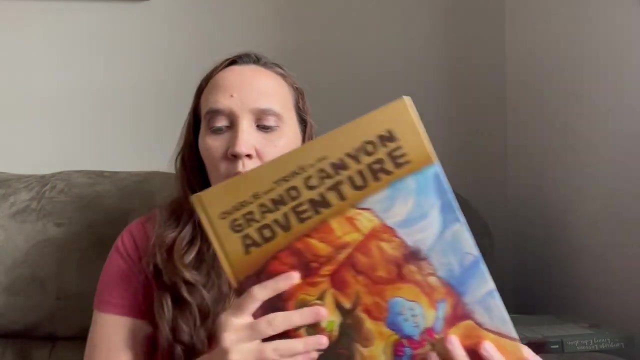 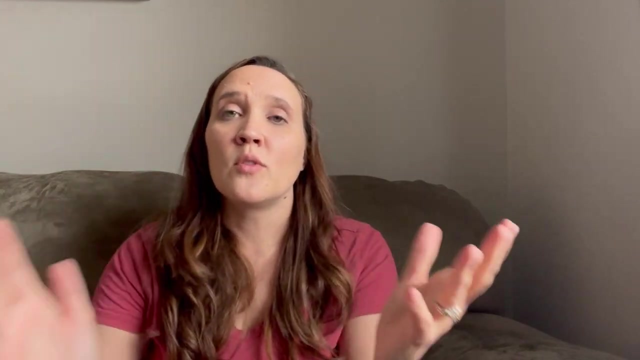 They are written in the student pages. The other thing it comes with is the book- Not Too Small at All- The Door to Salvation and Charlie and Trot in the Grand Canyon Adventure. So that is what it comes with. Now let's go ahead and get started with the pros and cons, so that you can hear my review. 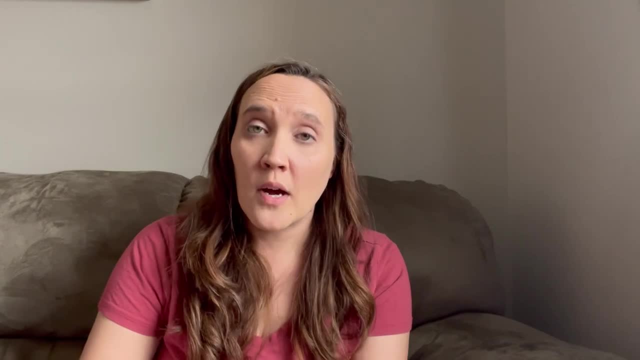 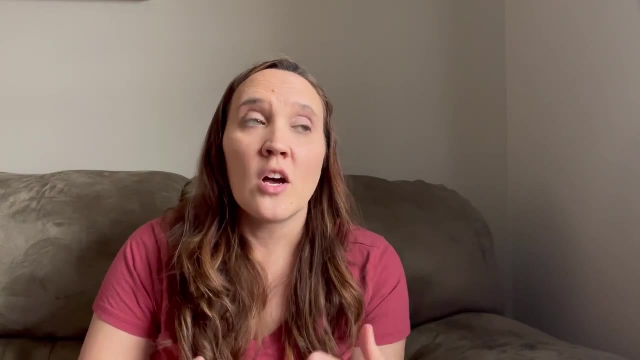 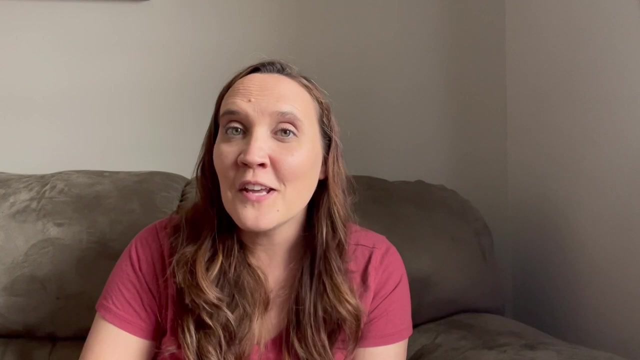 of this curriculum. So the first pro About this curriculum is something I already mentioned- is that it is very open and go all in one and it is not super teacher intensive. It is very easy to teach using this curriculum. I would classify that as a definite pro, especially if you are a large family mom like me, and 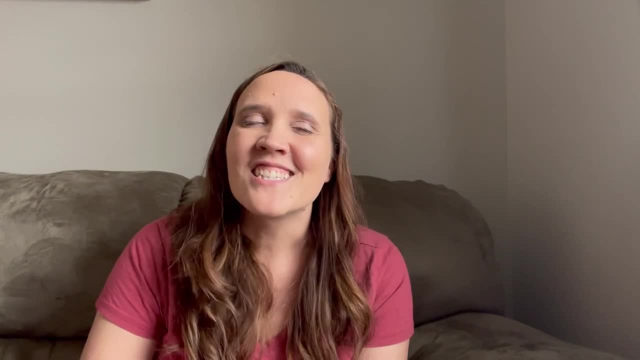 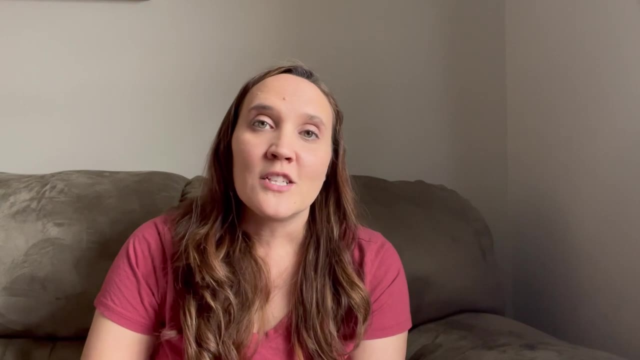 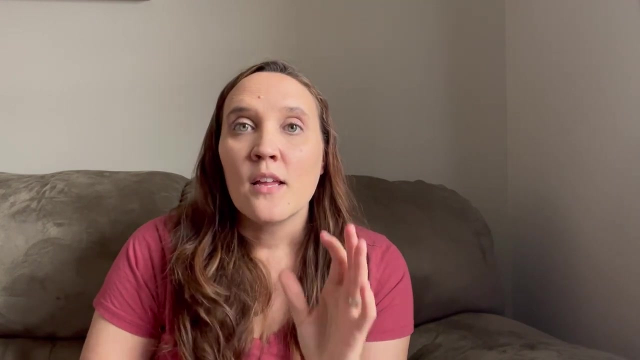 I am actually teaching three different children to read right now, So having something that is more easy to teach and open, to open and go is very appealing. The other thing, Something that is really nice about this curriculum that I have actually really grown to appreciate, is the fact that the reading in this they use phonetic symbols over the 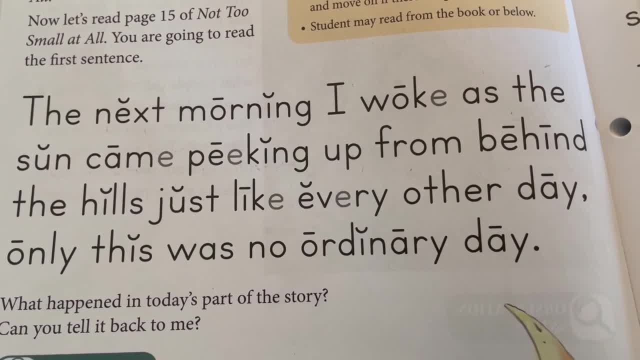 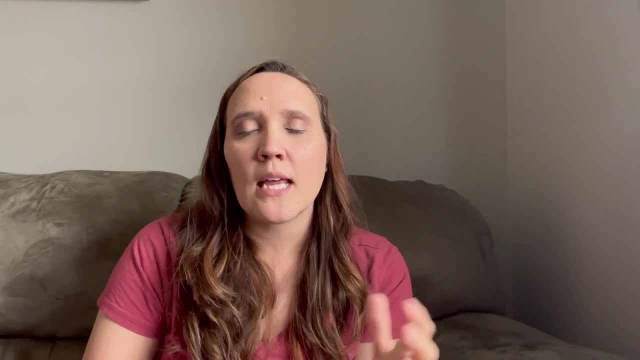 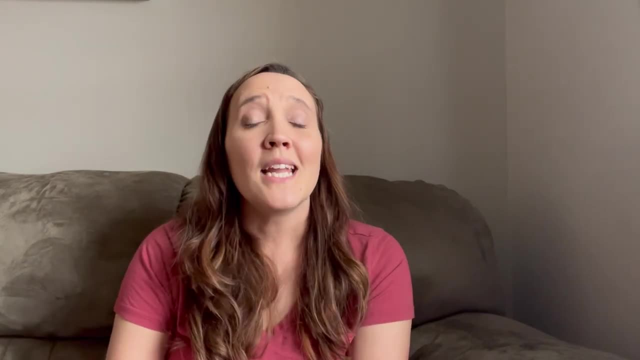 top of different letters so that your student can early on be able to delineate between short sound, long sound, different things like that. I found that extremely helpful, especially early on when you were trying to teach younger ones to read The next pro. 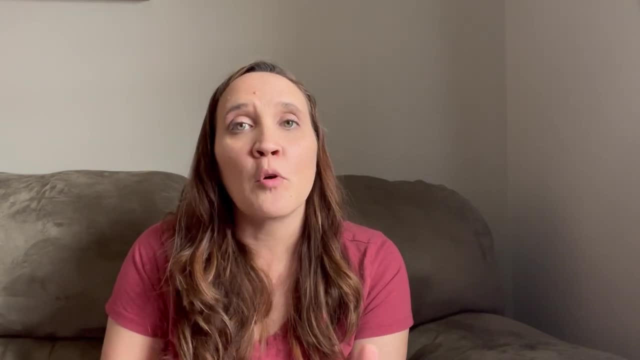 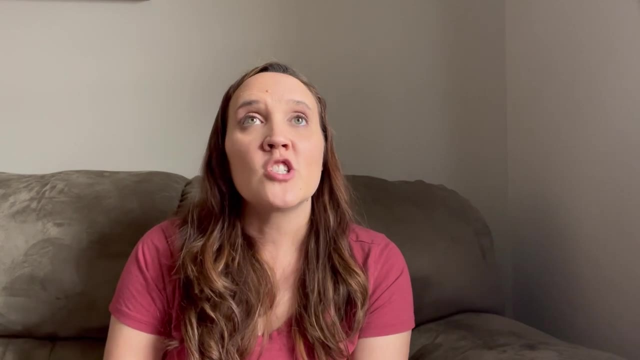 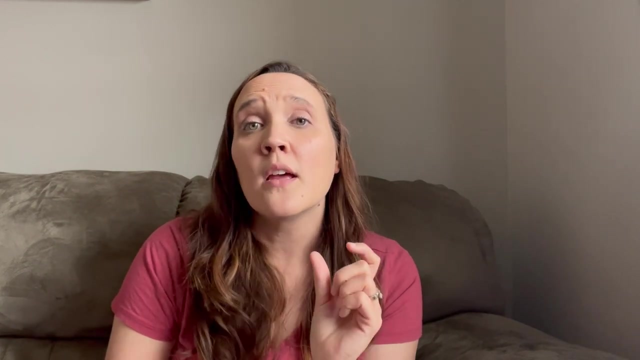 Of this curriculum is that it encourages reading more challenging passages and also more challenging words. I think that that is very important to challenge students, but at the same time, a con of that can be that for very early readers or for readers who aren't quite confident enough. 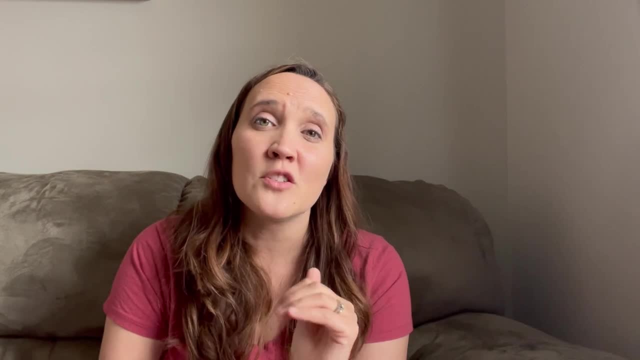 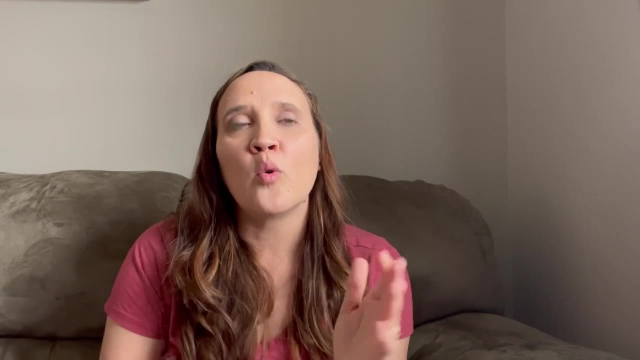 yet it can. it can be a little bit of a deterrent to reading. It can be a frustration in reading. So I think you just have to know where your child is at to figure out if that is going to be a good fit for them. 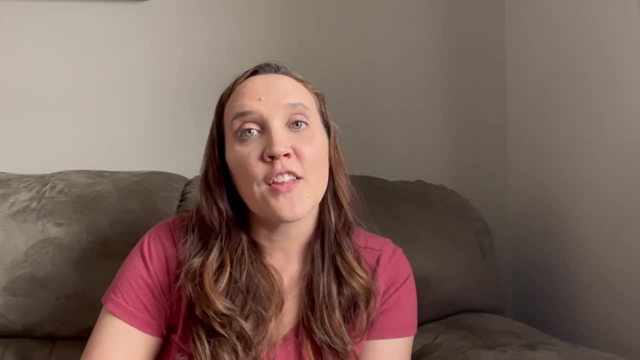 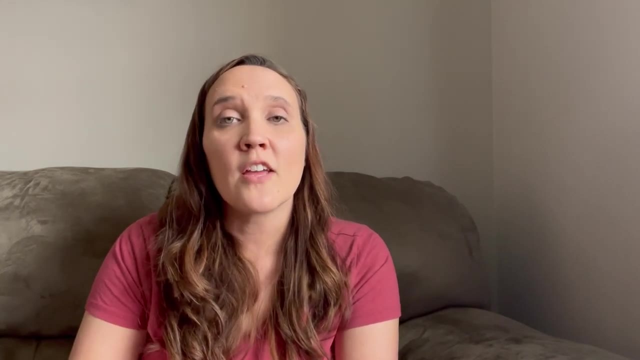 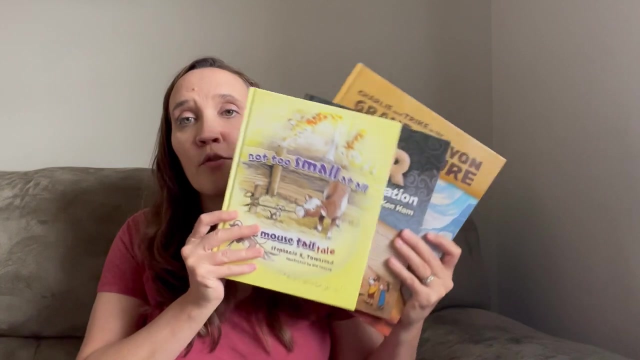 You don't want to overwhelm, but you also want to provide a challenge in there at appropriate times. The other thing that I really appreciate about this curriculum is the fact that it does have a very Christian focus. Even the companion books obviously are about creation and other truths about what we believe. 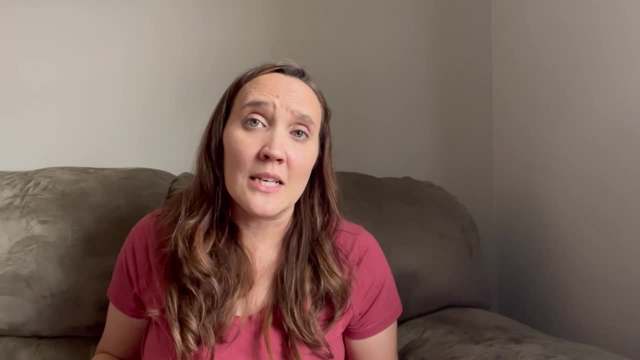 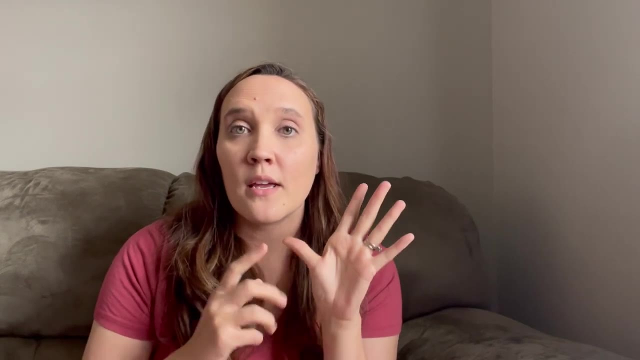 in Christianity as well, And they are very character building. Next thing, The other thing that I actually really liked about this curriculum is that I think it's on the fifth day of every unit in this curriculum that they do an activity that is a dictionary. 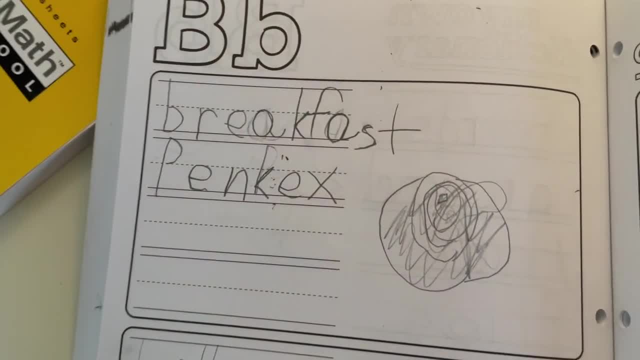 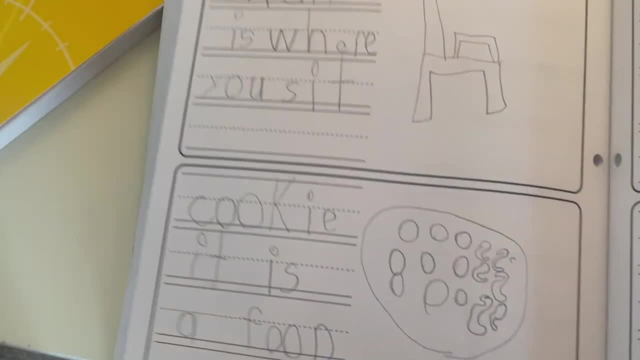 activity. At first I thought it was a little weird because it was words that they weren't able to read. However, I actually really enjoyed it and it is something that I definitely want to carry over in other curriculum that we use Um. it was just a great way to practice. 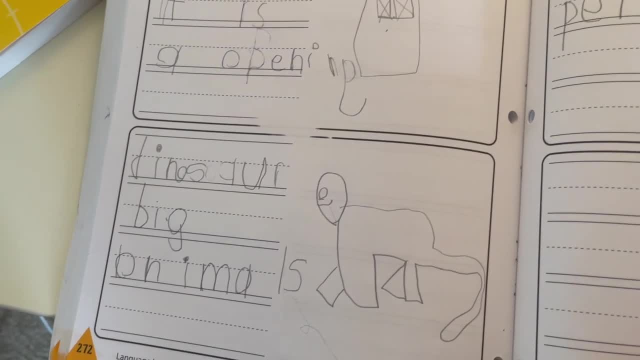 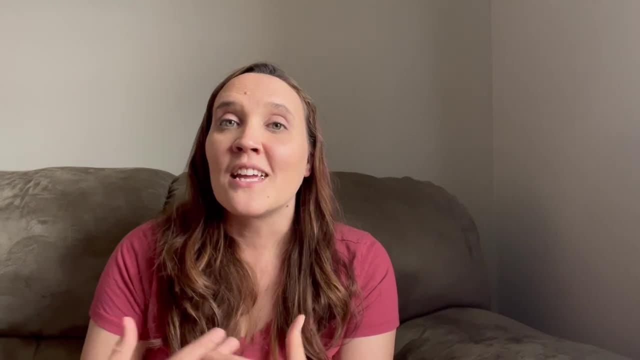 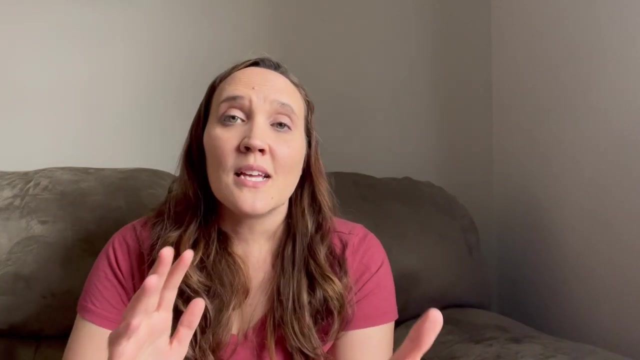 So practice those skills of writing um and also getting to draw and make their own dictionary, And also, without them realizing it, they are learning alphabetical order. So it's a neat little activity that is included in this curriculum. Now, this next thing that I'm going to talk about is both a pro, but then it also is kind. 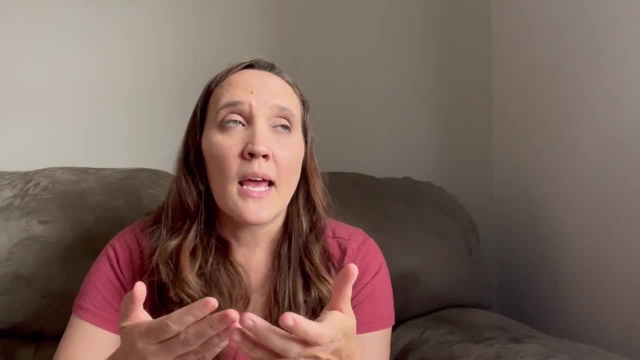 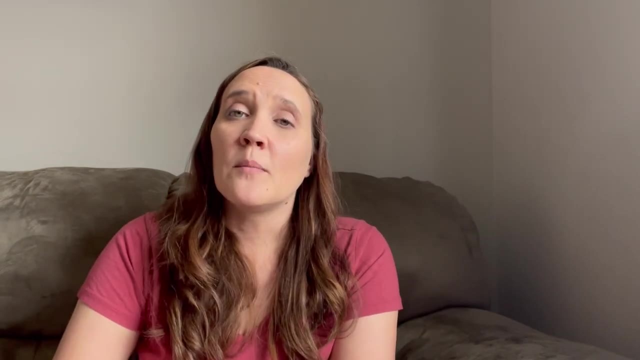 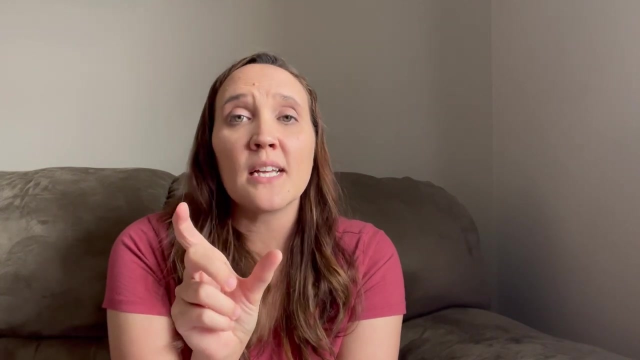 of a con Depends on which side of the spectrum that you're on and, um whether or not your child falls into one of those categories. So the lessons for this curriculum are relatively short, which can be a pro, because it can mean that you are focusing in on a specific goal for each lesson. 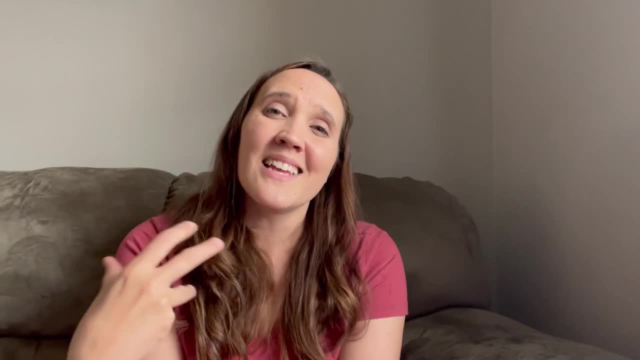 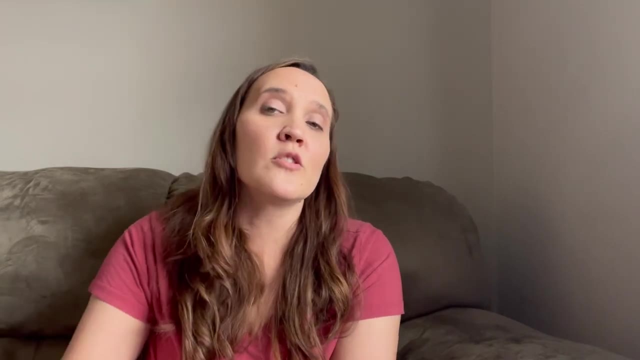 But sometimes those lessons are so short and concise that they lack the depth that some students are going to need, um, and the repetition that some students are going to need in order to have mastery of the phonics skills that are being taught in that lesson. 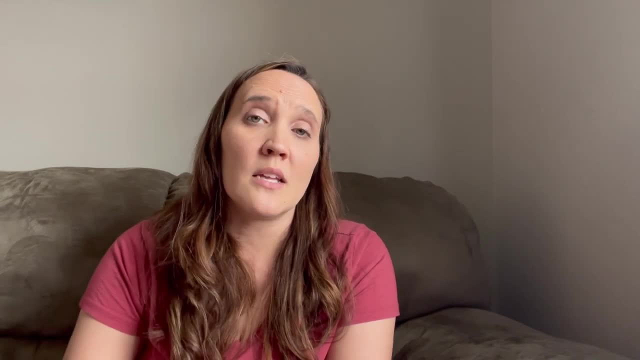 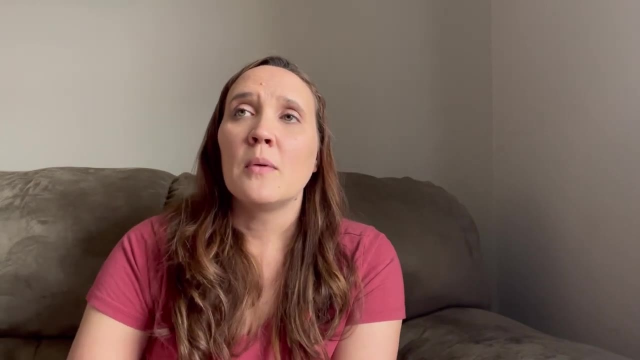 This is what ultimately led to us changing curriculum With my son that was using this. So we got about halfway through this curriculum and it just became very taxing for him because there wasn't a lot of depth and Tom spent on mastering those special sounds different. 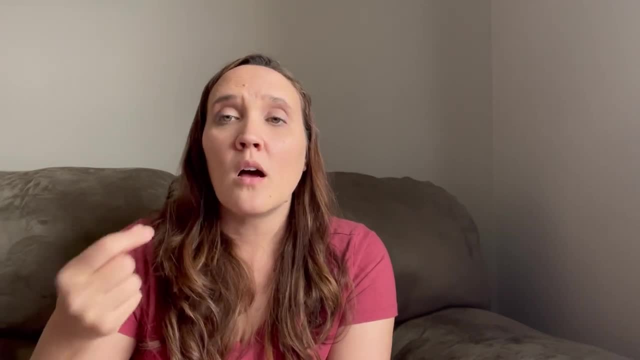 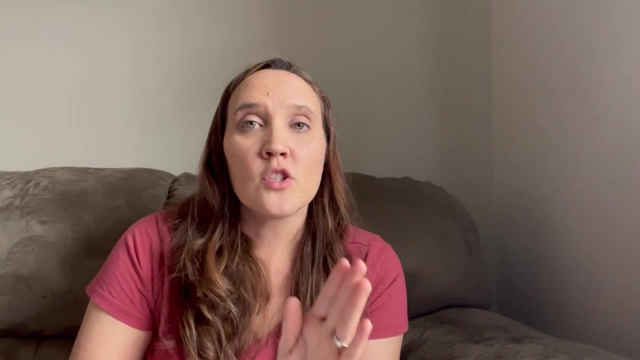 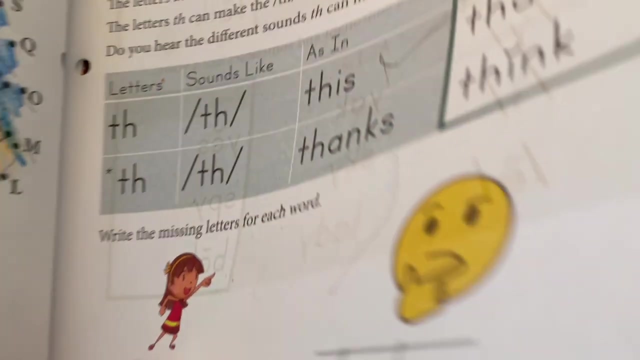 diagraphs and blends and things like that. There wasn't a lot of depth and Tom focused on mastering those. It felt like the curriculum was teaching new special sounds constantly, Okay- While he hadn't mastered the ones that were taught previously And he was trying to master a new set on top of that. 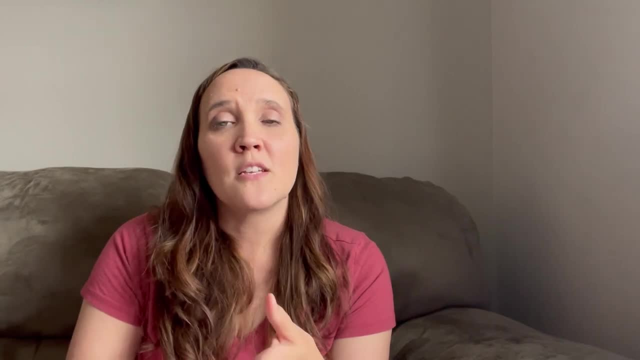 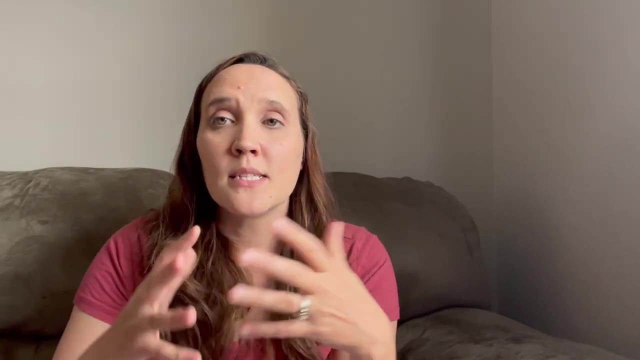 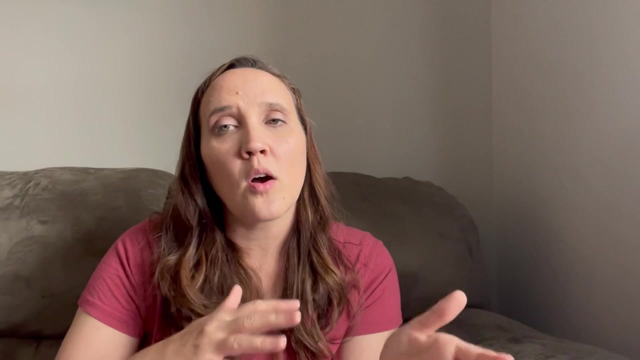 So it became a little bit of an overwhelm for my son specifically. He is not a lagging reader, but he is not a quick reader either And, um, I would consider him pretty average, especially for first grade level. And so because of that I I saw him getting a little frustrated, sometimes having a hard. 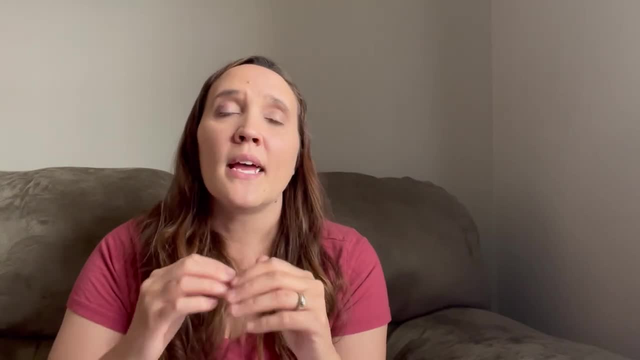 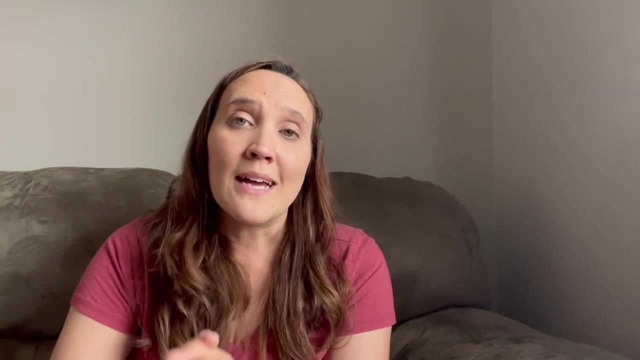 time remembering what some of those special diagraphs were, Um, but he was able to master them, Yeah, And so I just felt like he needed a little bit more depth and opportunity to solidify and to master those different sounds, And so that is why we ultimately switched from this curriculum. 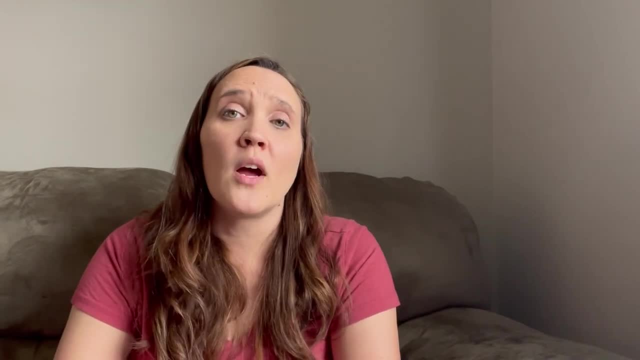 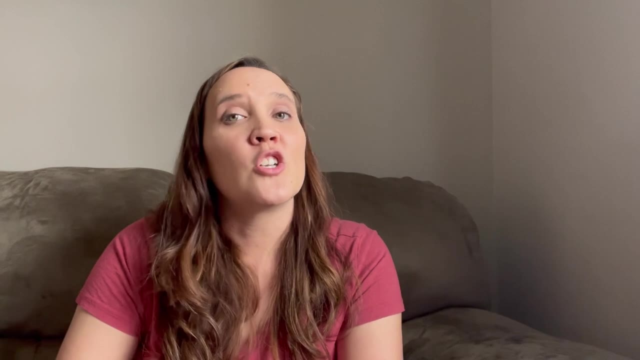 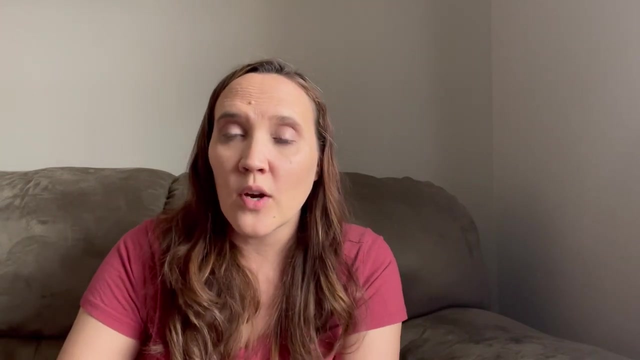 However, I could see this curriculum working very well for other children who are swifter learners in reading um, that don't need the constant repetition and who pick up on it pretty easily. In fact, my daughter is one of those readers, And while she is not using this curriculum, she's using one that moves a bit swifter, though. 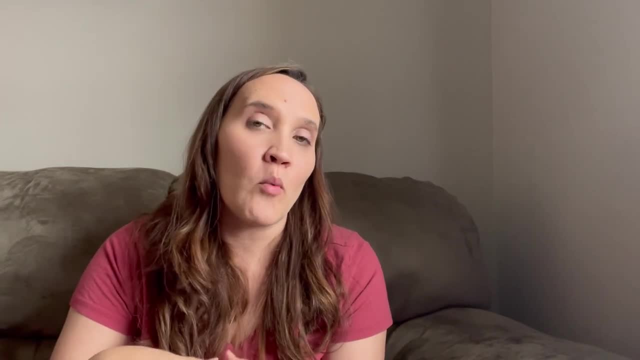 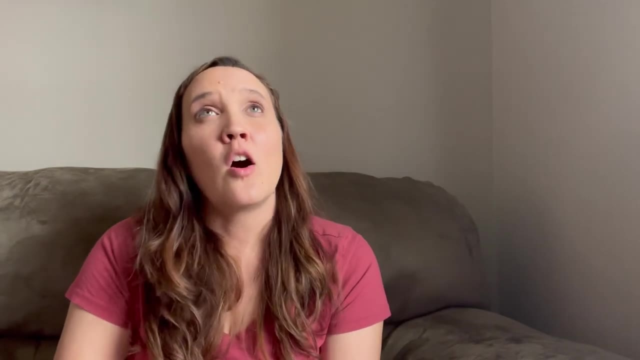 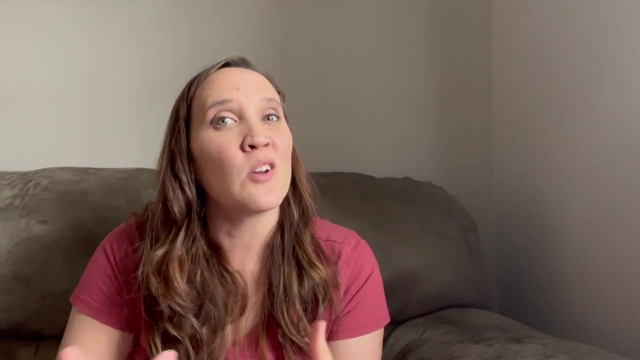 Um this. I could see this curriculum actually working quite well for her because she doesn't need that constant repetition and mastery opportunity. So again, a con, as I stated, can be that it does move rather swiftly And in our case that was a con for us because it wasn't a great fit for my son, who needed 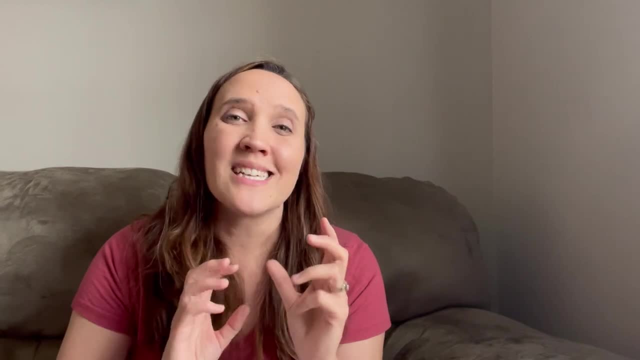 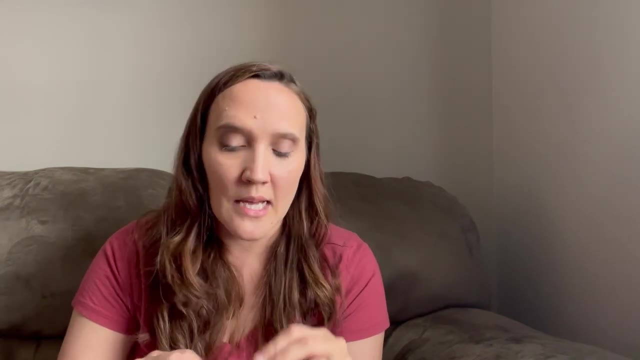 it to be just a little bit slower, a little bit more focused And to Provide a little bit more review and opportunity to really solidify the concepts. So, as I stated, this was not exactly a great fit for my son, but I do know that it works. 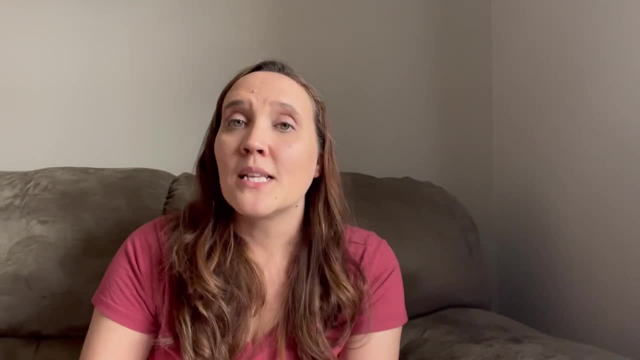 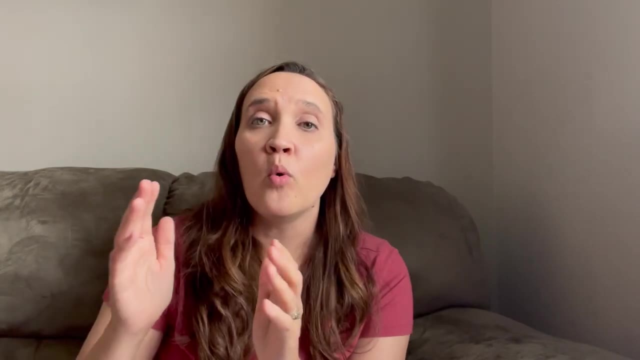 very well for others with the information that I've given. perhaps that can help you in making your decision of whether or not you need to focus more on a more mastery phonics based program or be able to use something like this Now for my son. we did move on to a different reading curriculum.